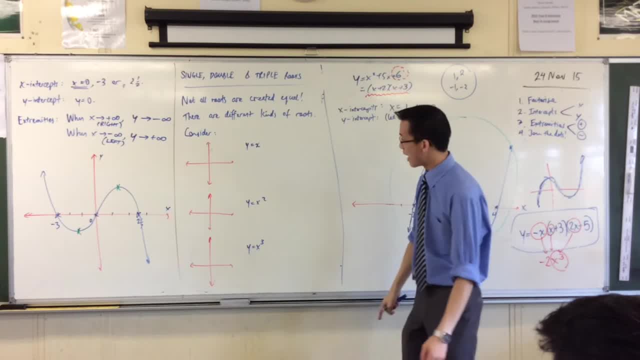 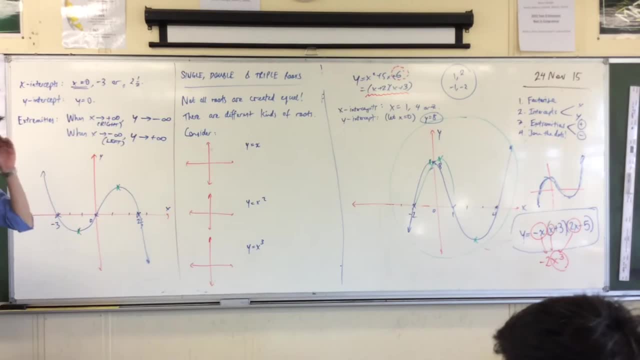 Now to illustrate how they are different. we are going to look at these three example curves, because we know how to do all of these curves. We know what they look like. They're very simple, okay. So you can see, I've just got a small set of axes for each one. We're going to draw it and then we're going to make some statements about it. okay, So y equals x. if you had to describe y equals x- the graph of it- verbally to someone, how would you describe it? What would you call it? 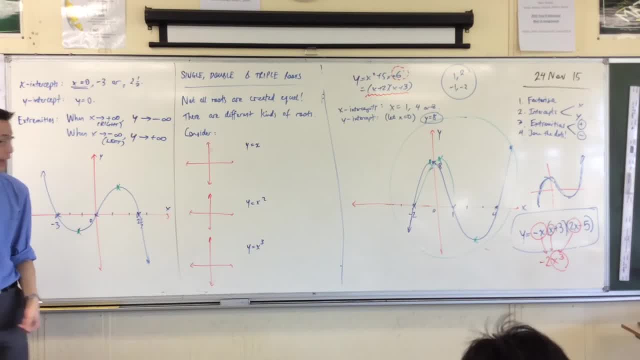 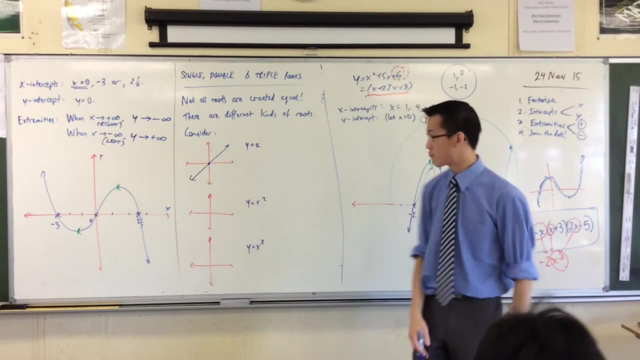 It's linear, It's a straight line, okay, Passes through the origin and it's increasing, It's going up, okay. So I'm going to draw that and you can draw one as well. It doesn't have to be beautiful, okay, But this you can see, there's a root at the origin, right, Is that? okay? No big deal. We call this a single root. 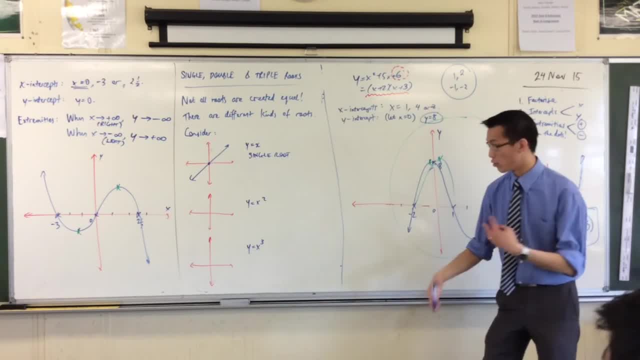 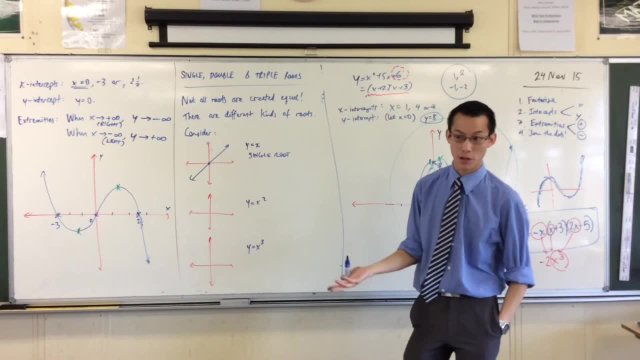 We're going to label all of these, okay, And then I'm going to add some more language to describe what's going on. okay, Y equals x squared. Again, it's a graph you're super familiar with. It has a special name. It starts with a p. It's called a. 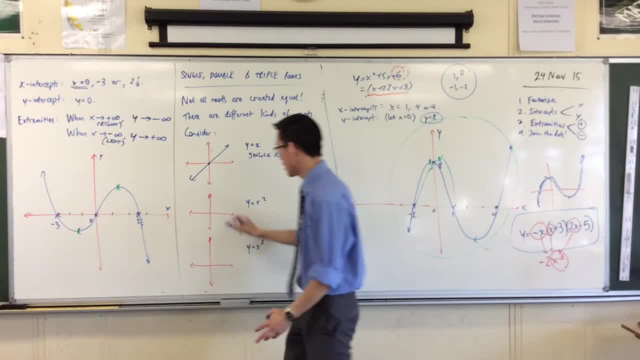 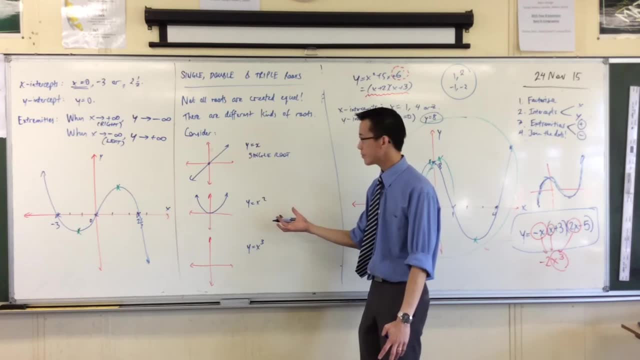 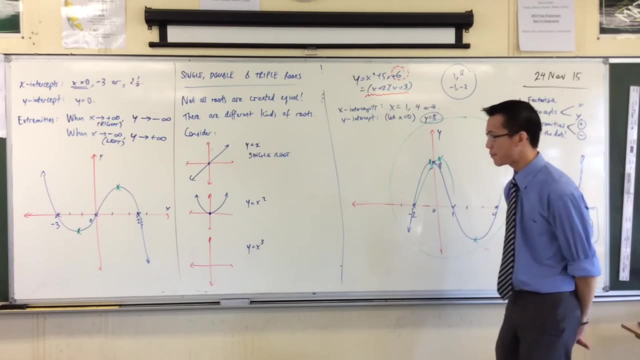 That's what I meant to say. It's a parabola, right? So again, let's draw this right. It comes down, it stops and it turns around like that. Now again, y equals x squared. it has a root at the origin, okay, But can you see, it's a different kind of root, right? Because you know, when we had a look at this, it's like quadratics: We expect them to have a root at the origin. 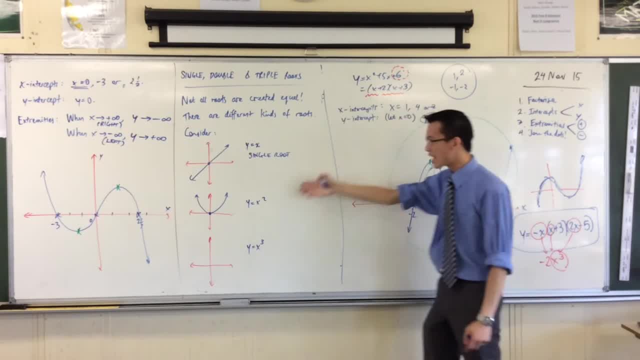 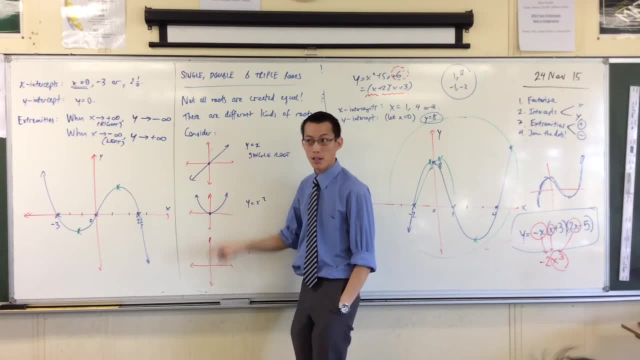 We expect them to have two roots: One here, one here, right? Well, this guy kind of has two roots as well. They just happen to be both at the same spot, right? They're both at x equals zero. So, being that there are kind of two sitting on the same spot, we call these double roots. 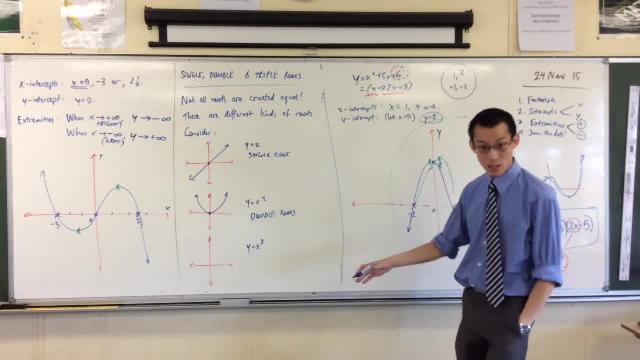 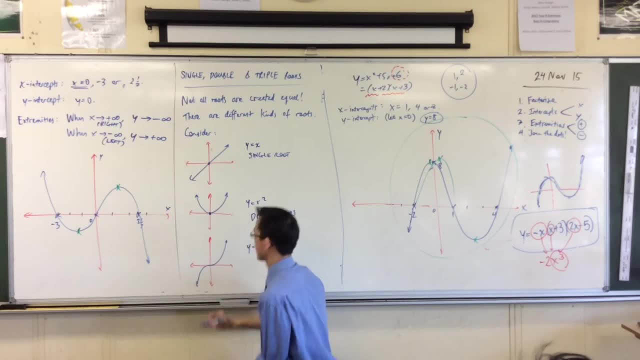 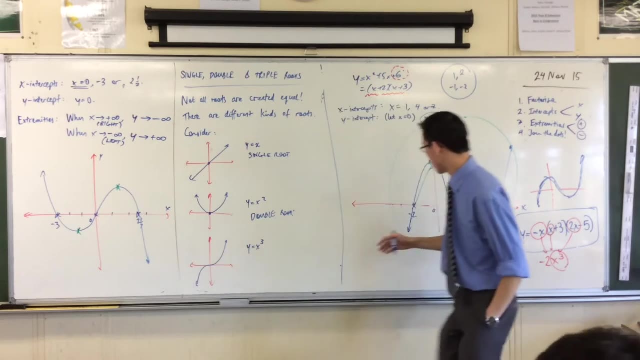 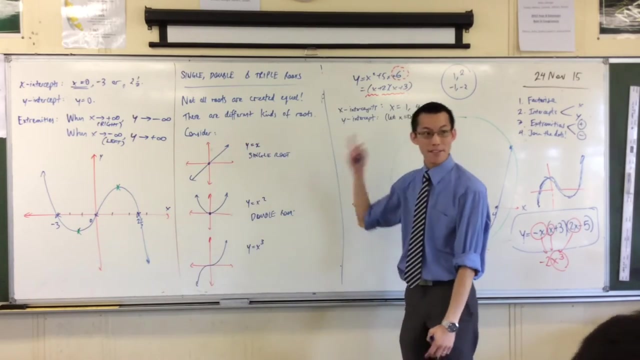 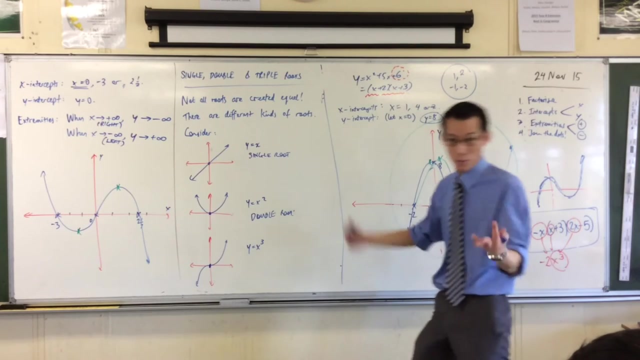 No imagination for what's going to happen next. right, We've seen this cubic before. okay, Again, coming from the left, it starts at the bottom, it goes up and it comes up like that. okay, Now, this is called a triple root because, again, a cubic. you know, like this cubic, or like this cubic, we expect it to have three roots. And this one does have three roots. They just all happen to be at the exact same spot, at the origin, at x equals zero. So, being that there are three of them, we call it a triple root. 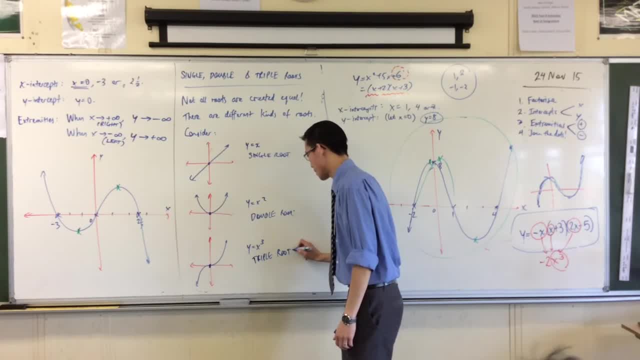 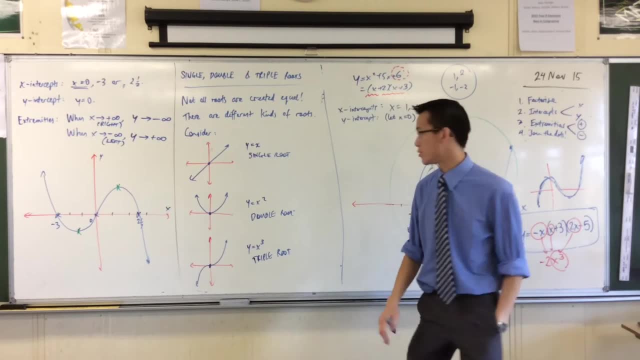 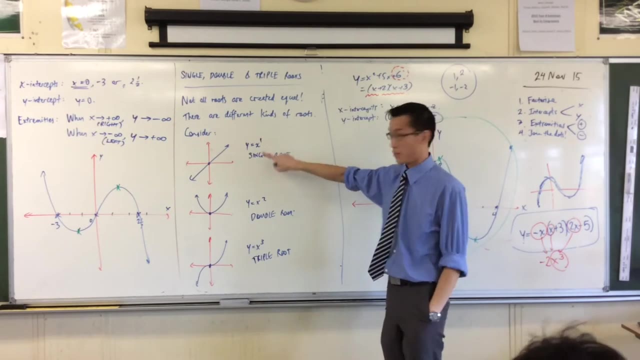 Now you can see a few things. Number one: this language here. right, The single root, double root, triple root. What it's really referring to is the degree of the coefficient, sorry, the degree of the polynomial right. If you've got x to the one, you've got a single root. If you've got x to the two, you've got two roots. If you've got x to the three, you've got three roots. okay, 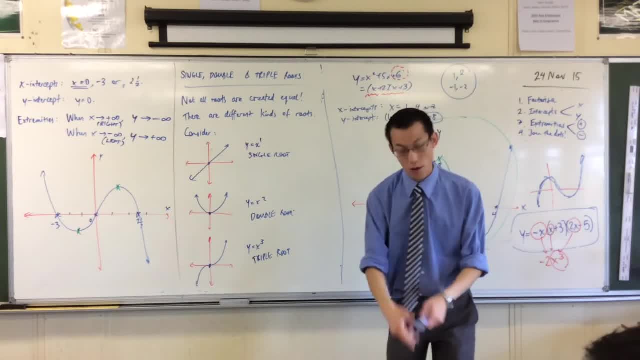 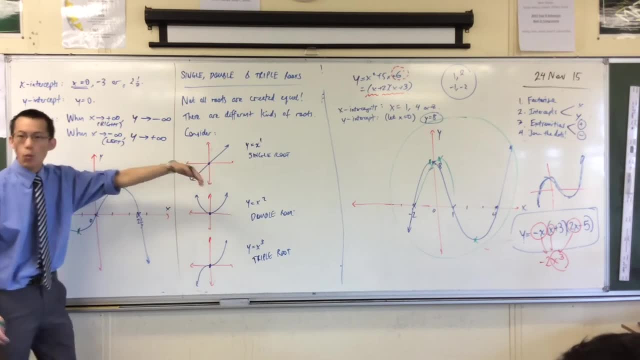 So that's where that language comes from. right Now, how would we describe verbally what's going on? okay, I've got some words here that I hope will help you articulate what's happening. right, This root here. what is the graph doing as it passes through the root? Well, it just sort of cuts straight through the axis. 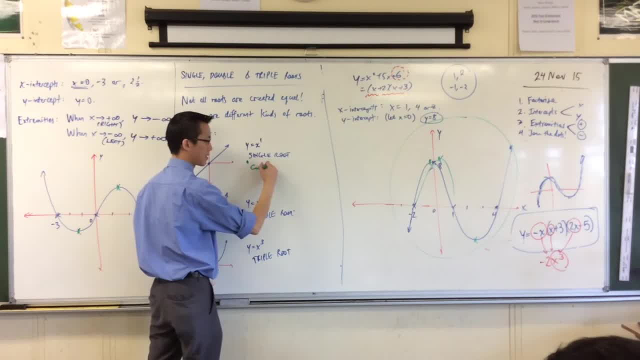 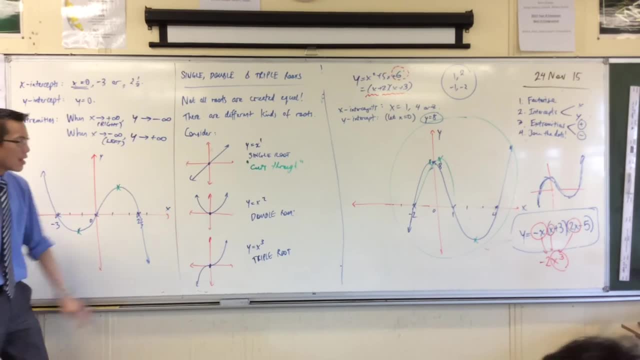 See that It just slices right across. So in fact, that's the way I say it: It cuts through and keeps on going uninterrupted. okay, Now, when you have a look at this one, it doesn't just cut through, right? In fact, it does something quite different. 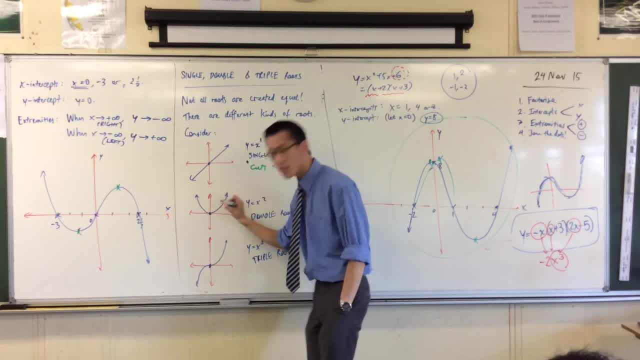 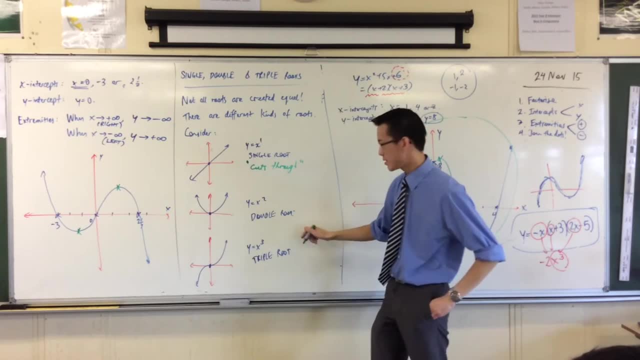 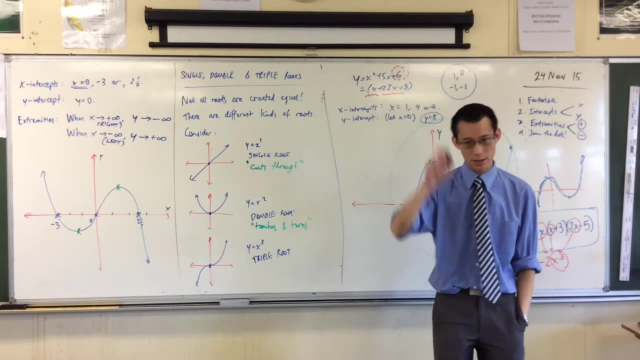 It comes down, it slows down, it just touches. Do you notice that It just sort of hovers there and then it turns around, okay. So the way that I would explain this is that it touches the axis, It turns. okay, That's what a double root is doing. You see, it comes down, it stops and then it goes back up, okay. 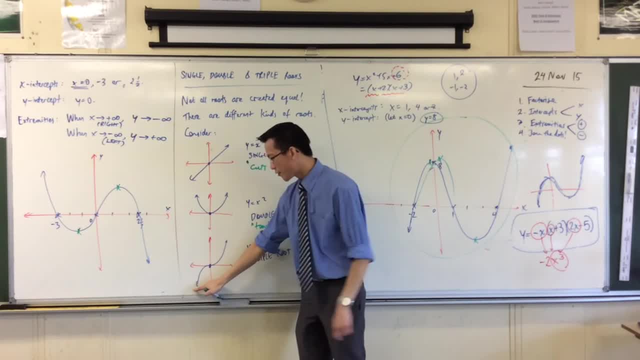 The last one, a triple root. right, It's starting from one direction. It stops there and pauses for a minute, but it doesn't turn around like the double root does. In fact, it just keeps on going after it's paused there. okay, So this cuts through, this touches and then it turns. 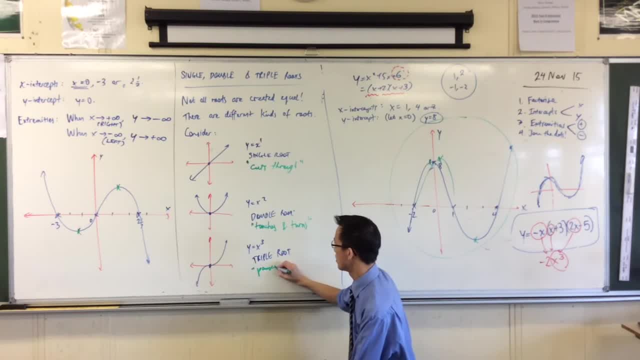 This guy, the way I say it is: he pauses And then he passes through Right. He keeps on going in the same direction that he was going before- right. In this one he's going up right. So he goes up, pauses and then he keeps on going up right. 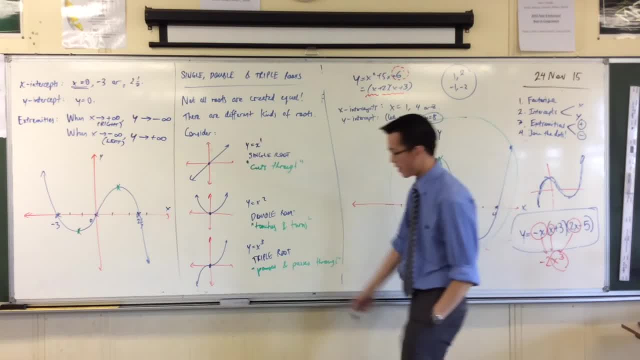 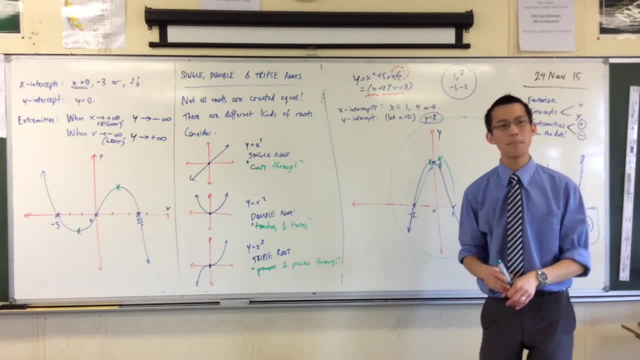 I could just as easily have had a triple root that went the other way. that's coming down and then he pauses and then he keeps on going down. So these three categories of roots, we can combine them in all different kinds of ways and get different kinds of graphs. 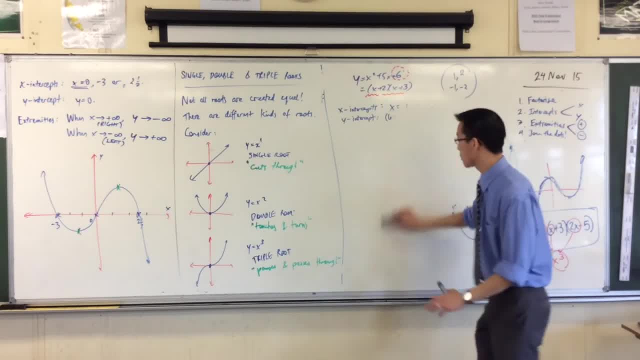 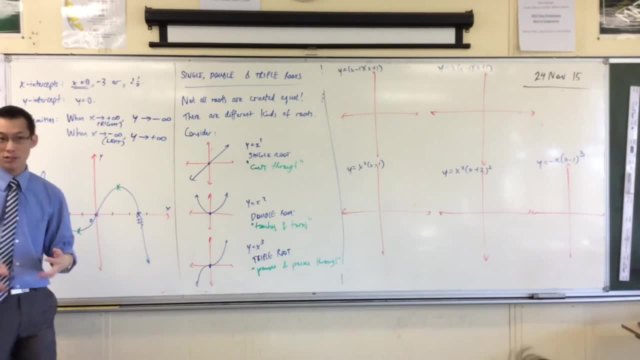 So let's quickly do some very, very brief examples. These are all going to be like kind of um, quick and dirty versions, so they don't have to be very detailed, okay, But I'm going to give you quite a handful, So the first two are really easy. but just I want to see that you understand this idea here. 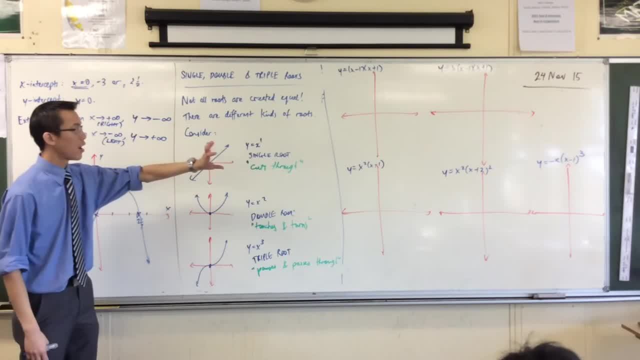 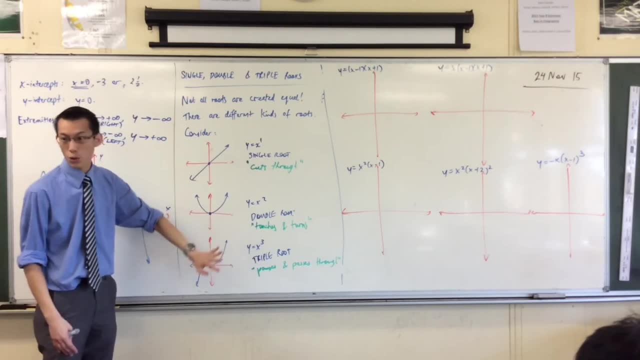 um, even from the most basic foundations, right? So I'm looking for when I have, these are all factorized for you. okay, I'm looking for the roots, and whether they are single roots, double roots or triple roots, right? 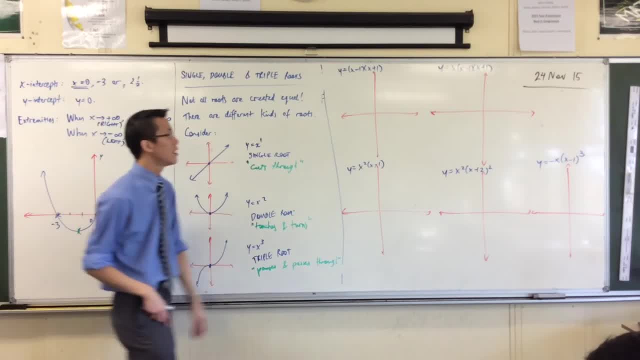 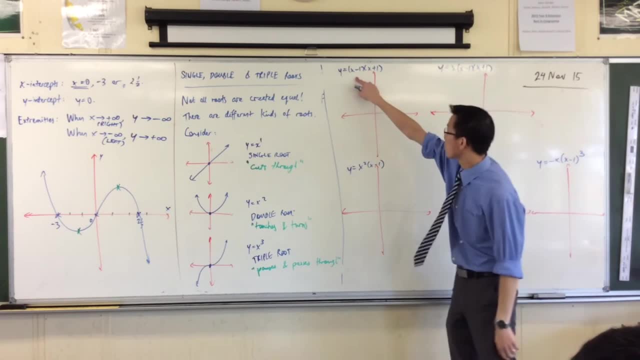 Because then I can characterize them and I can talk about how they're behaving, right. So up here, have a look at that guy. How many roots does he have? He has two, here's one, here's another one, and what kinds of roots are they? 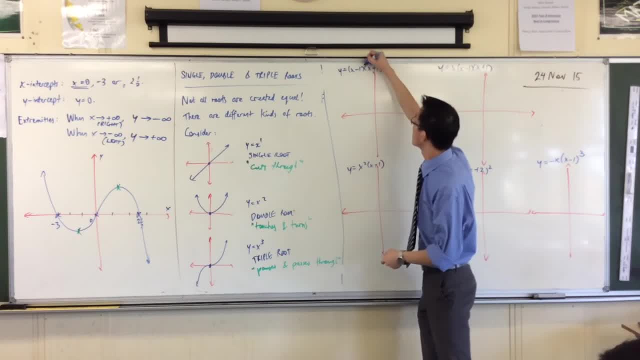 They are both single roots. Do you see that? I mean I could write one and one there, okay. So in other words, at x equals negative one and x equals one one negative, one, right? The graph is just going to cut through the axis right Because there's two single roots, so that's easy enough. 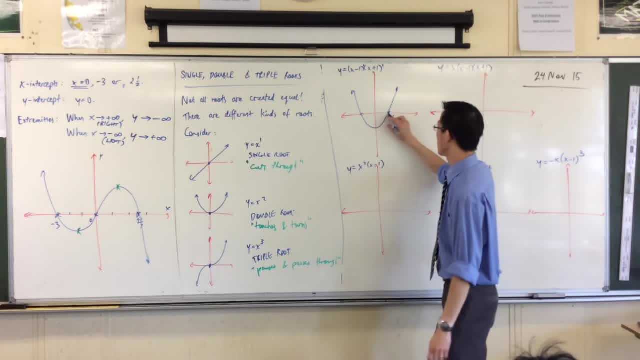 This is a parabola. I know what these look like. no big deal, okay, Minus sorry. positive one and negative one. Okay, So it just cuts through. Again, having a look at this: how many roots are there? 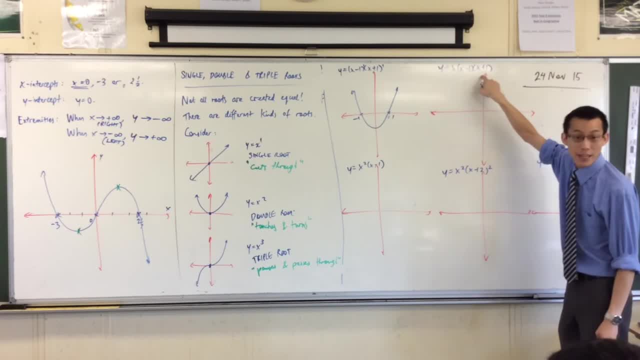 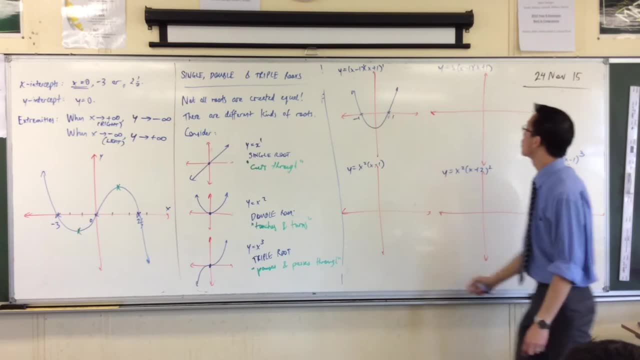 There are one, two, three, and each of them is a single root. Do you see that, Like, the power attached to each one is a one? okay, So when I look at the numbers here, I've got negative one and zero and one, and I'm just going to slice through. 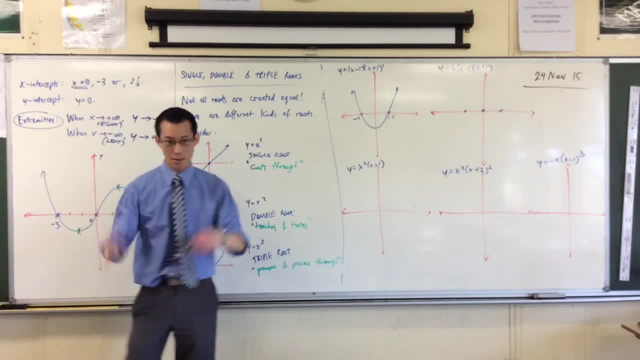 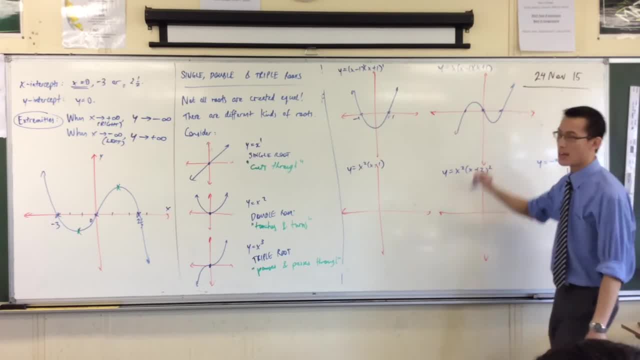 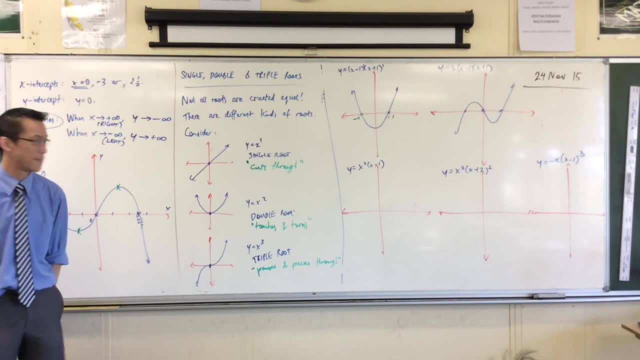 I'm going to slice through, slice through, slice through. There's those three single roots, and each time it cuts across the axis and it doesn't stop. Okay, But here's now where it starts to get more interesting. Have a look at this guy, right? 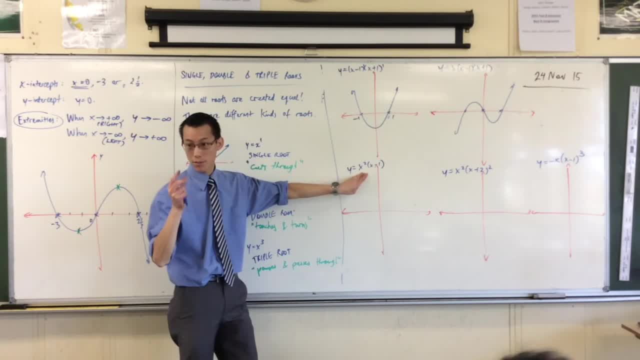 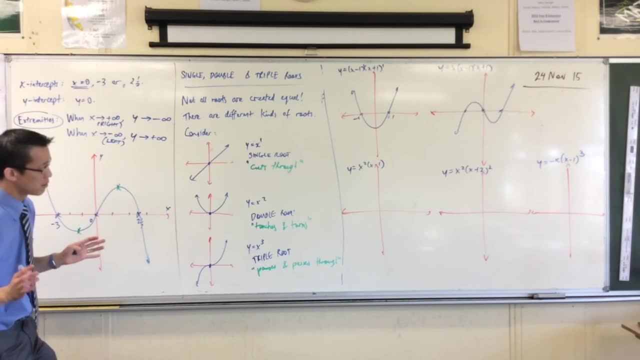 You can say, like, when I ask the question, how many roots are there? You can say this in one of two ways, okay. You can either say: oh, what's the degree of the whole polynomial? What's the degree of the whole thing? 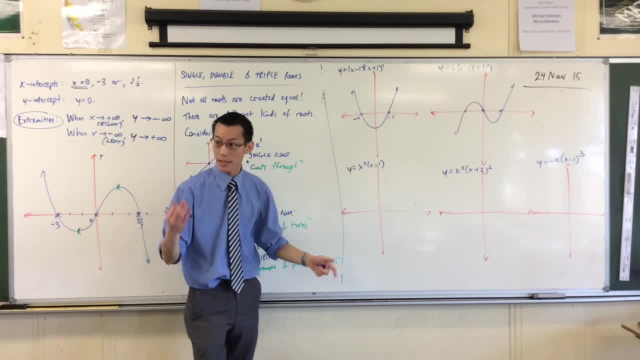 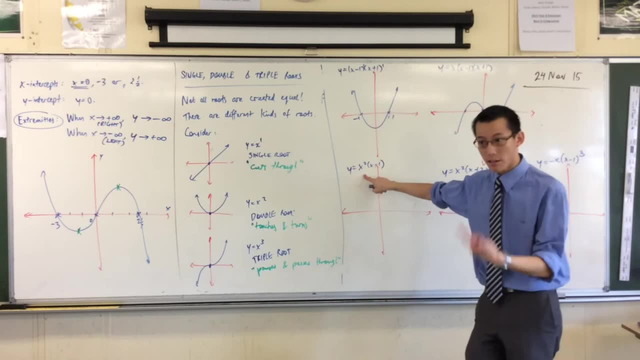 Careful. Two Oh three. Now you see a two there, but the actual whole degree is three, right? Thanks, man. Do you need me or do you Just double it? Okay, So you can see. the whole thing is degree three, right. 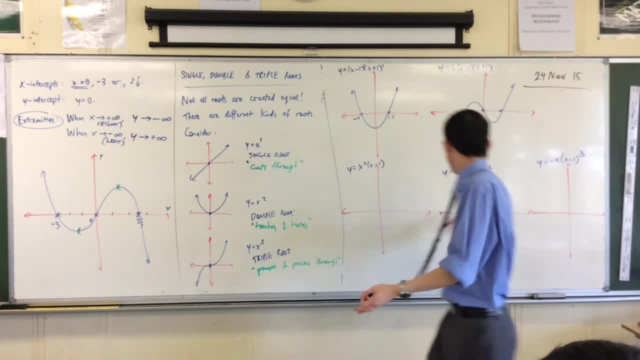 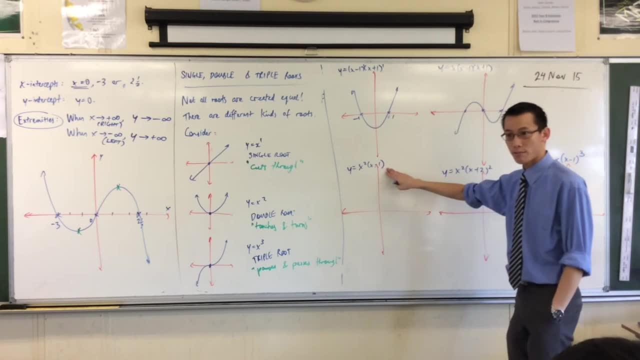 So I could say there should be three roots, right? That's what you expect of a cubic. Look here's one, right. But another way I can say it, using this language here, is that there are two roots: This is a single root and this is a double root, right? 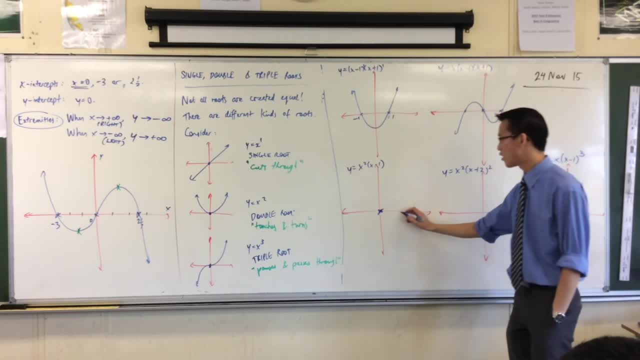 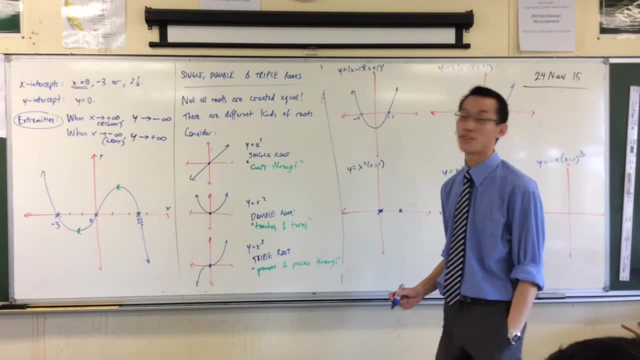 So I've got one at zero. There's my double root right there, and then I'll have one at one. Someone in particular looking for one? No, I'm just counting numbers. Oh sure, No, no, no, Yeah, yeah. 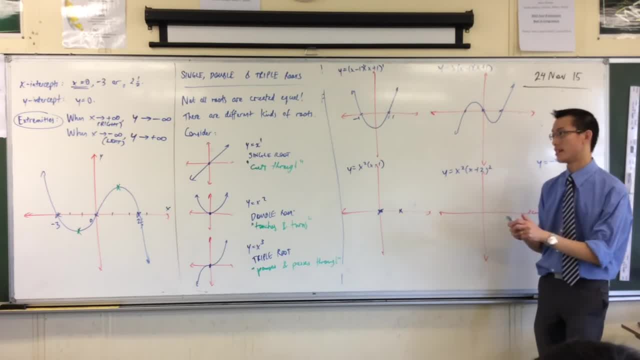 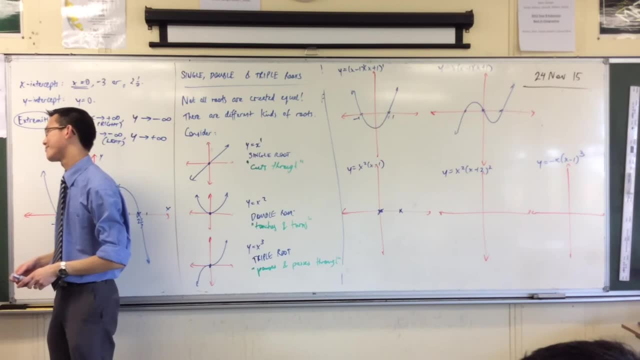 Can I quickly ask you something? Yeah, of course. Are you on key period one? Yes, In here. Yes, A kid is going to come here at ten past nine who I was going to have sit in test period two. However, it's going to be a shortened period and he needs 45.. 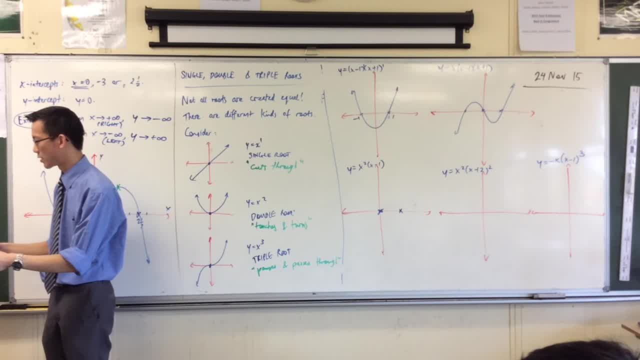 Could you get him to do that? Yep, Ken Payne. Yeah, Yeah, that's fine. Do you need it? You want me to show his name? Well, I wanted a timer, That's all, Yeah, sure, Okay, that's fine. 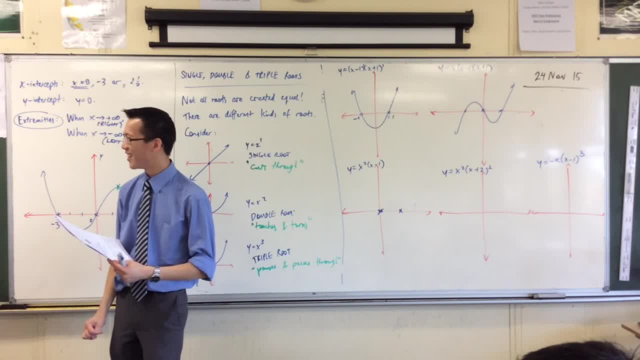 Oh no, my phone's down at the back. If you could just tell me what time it says on that clock at the time, I'll time it from there. Okay, Because I'll have him period two. Oh, okay, sure. 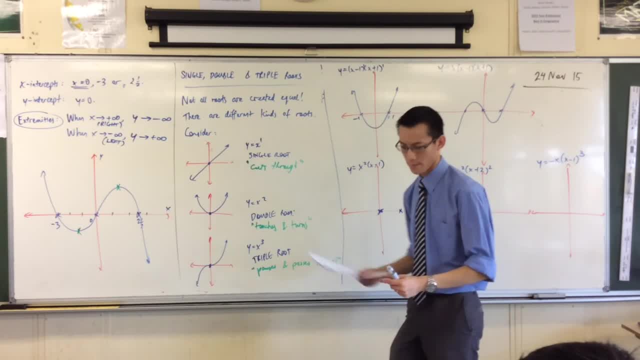 I'll be here. That's what it'll be, Is that okay? Oh, I see. Yeah, that's fine. Yeah, because it'll go through both. I'll take care of it. It's already dropped, No easy. 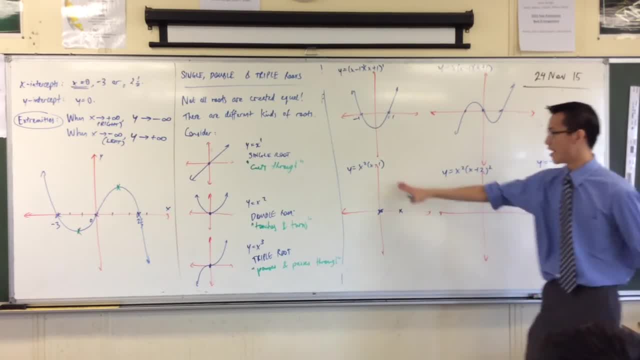 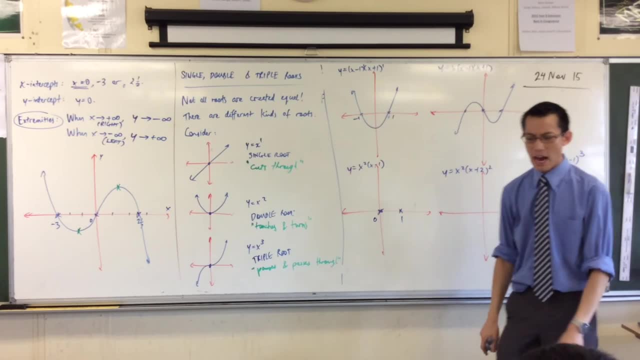 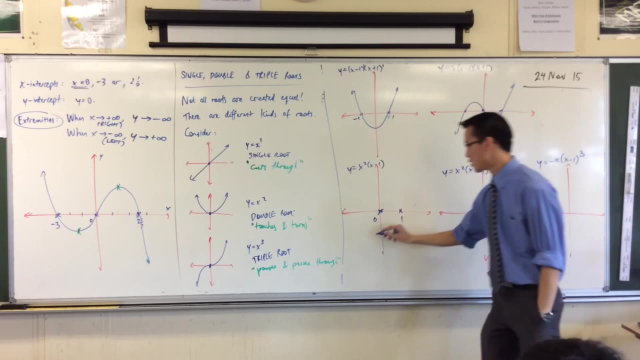 Okay, guys, I'll quickly finish before you head off to roll call. okay, Now, double root at zero. You should label that A single root at one. Now, what's this thing going to look like? right, Well, I know, by doing my extremities I'm going to go negative and then positive. 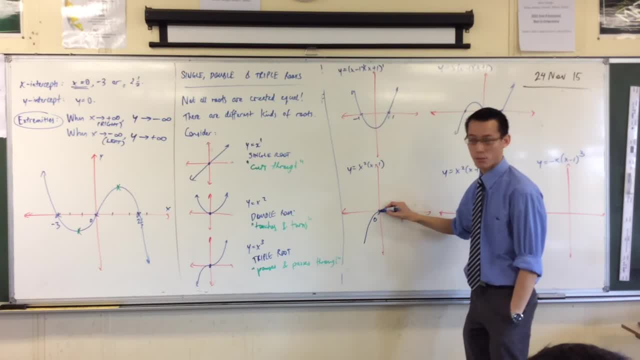 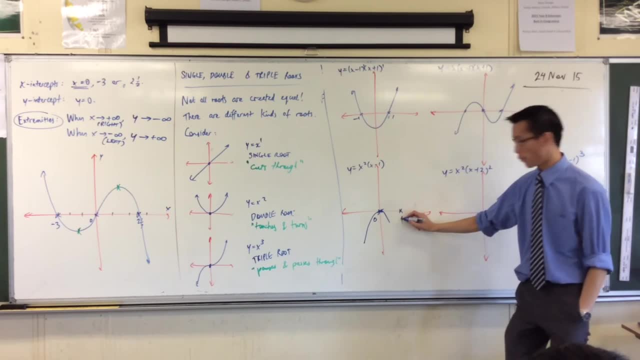 So I'm going to come up, I'm going to touch there, but because it's a double root, it touches and then turns around. It comes back down, right, But then he's got to come back up to this single root, right. 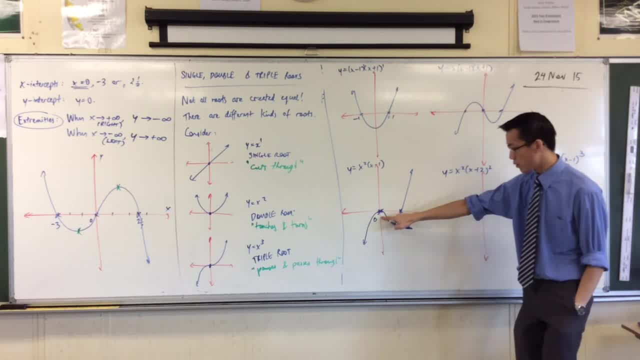 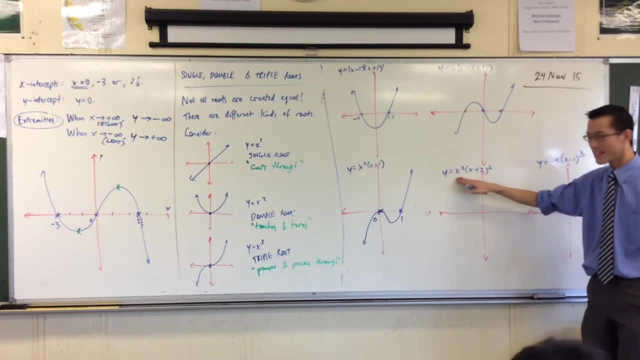 And then just blow through like that. You see that Double root, single root, Touches and turns, cuts through. okay, Keep on going. How about this guy right? How many roots are there? Well, I can either say there are four roots or I can say there's a double root there at zero.